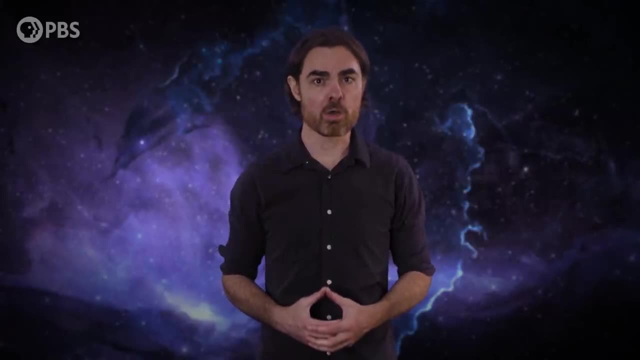 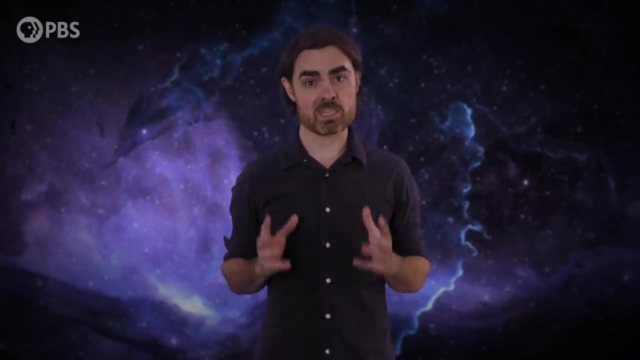 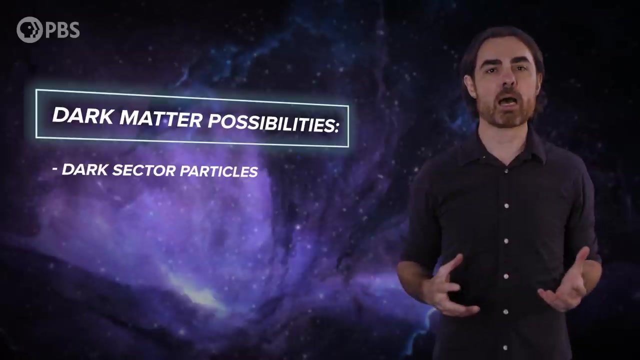 that we can see A dark universe that overlaps our own But so far is hidden from even our most ingenious experiments. Today we're going to open the gateway to the dark sector and see what we can find. When we talk about the dark sector, we typically mean a particle or family of particles that 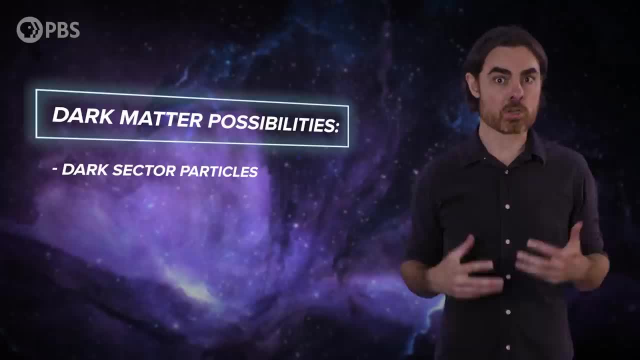 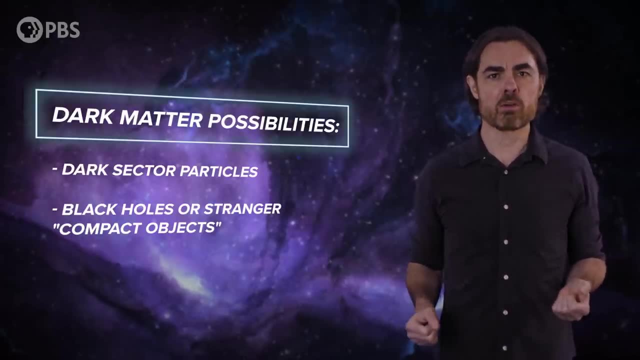 contribute to dark matter. Now, it's possible that dark matter is not particles. It could be black holes or failed stars or, even weirder, so-called compact objects. It might even be that what we perceive as dark matter is really a glitch in the laws that we use to describe. 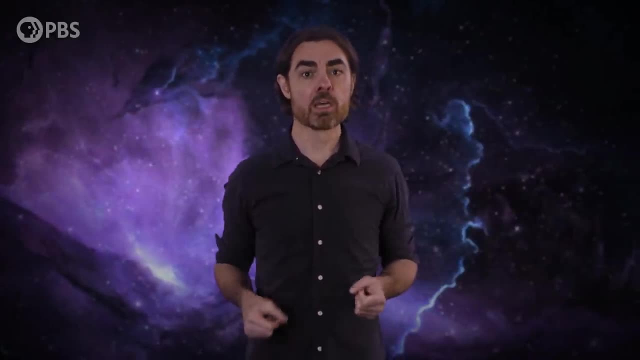 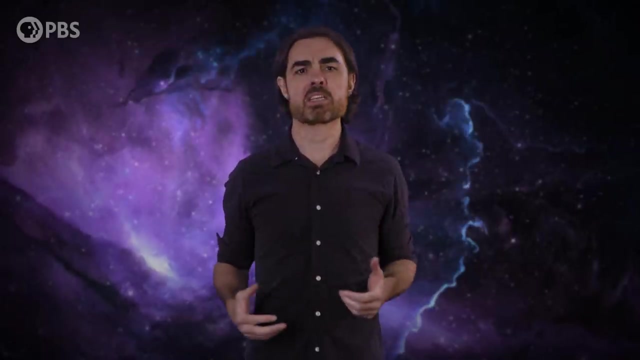 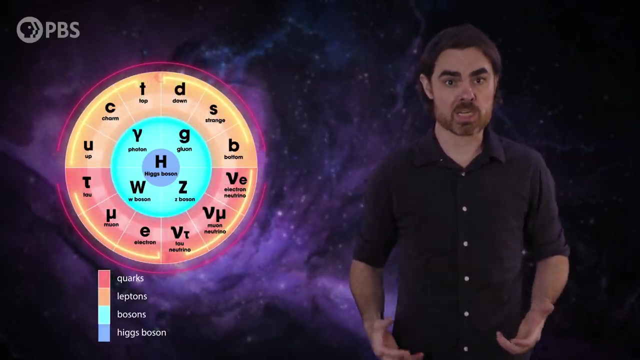 gravity. But those possibilities are for another time. Today we're focusing on the bizarre physics of the dark sector, So let's begin with what we do know. Our best understanding of the subatomic world is given by the standard model which describes the behavior of the known family of particles with incredible success. The visible universe. 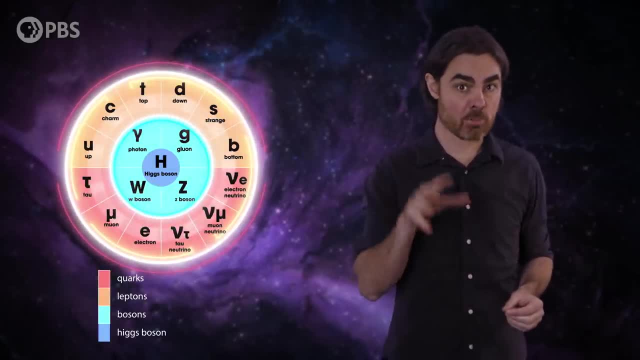 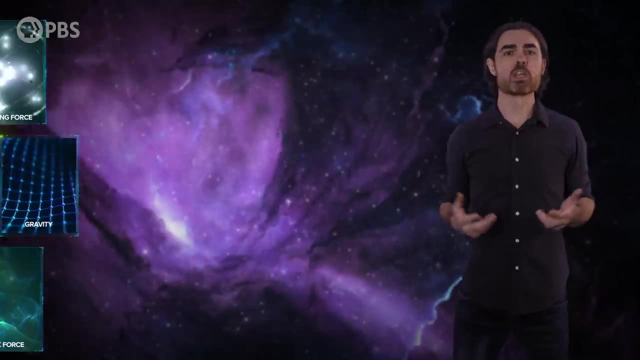 is made of these particles interacting with each other through the standard model forces – the strong and weak nuclear forces and electromagnetism plus gravity. In general, the behavior of the subatomic world is based on the idea that there are no forces. The behavior of a particle is determined by the forces it interacts with. 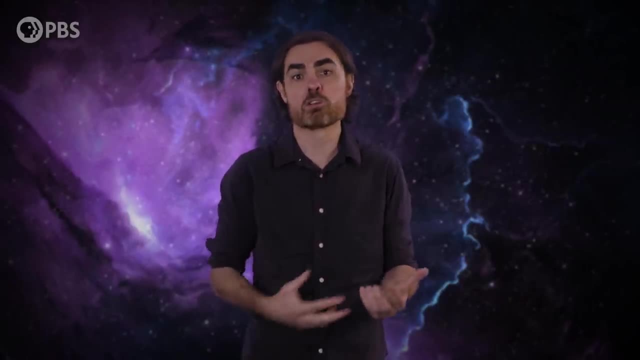 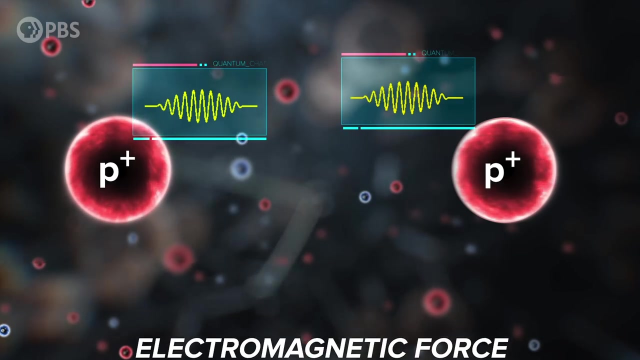 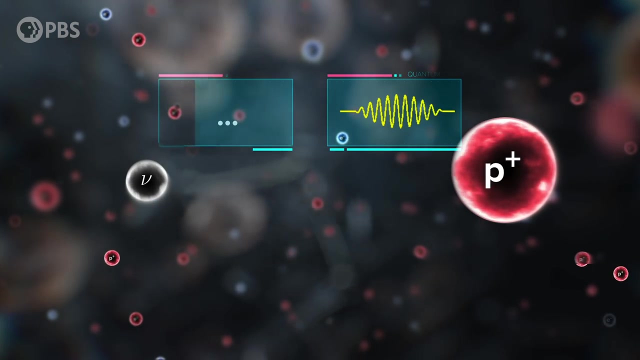 We can think of forces as the languages that particles use to communicate. Any electrically charged particle experiences the electromagnetic force and can communicate with other charged particles by exchanging photons. But for an electrically neutral particle like a neutrino, electromagnetism is a language it doesn't speak. Neutrinos are unaffected by that force. 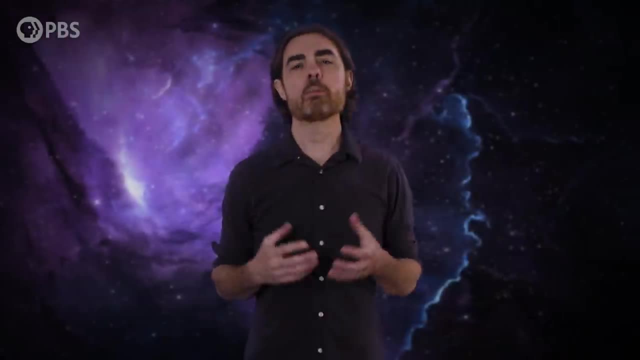 and so they are quite literally invisible to photons. The strength of a particle is determined by the force it interacts with. The strength of a particle is determined by the strength of its interactions with photons. The strength of a particle is determined by the strength of its interactions with photons. 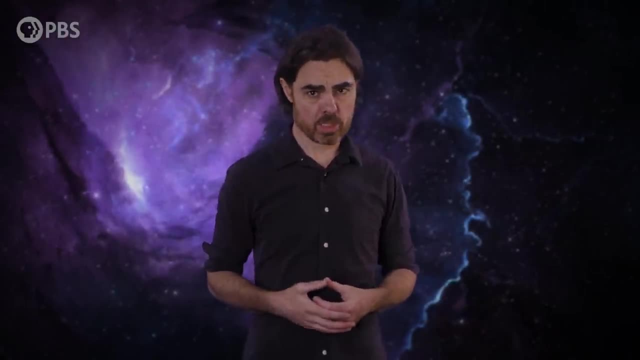 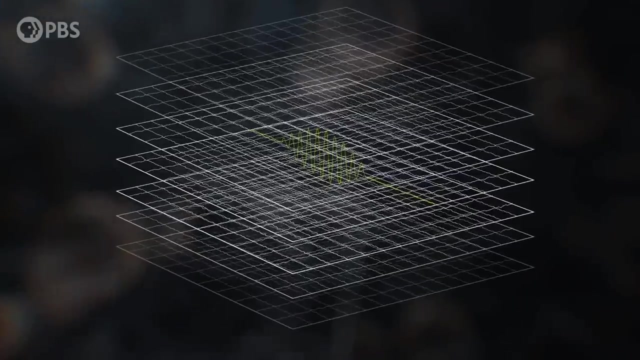 A more technical way to think about this stuff is in terms of quantum fields, where each particle and force is a vibration in its own field. These fields fill the universe, overlapping each other, and if a particle field is connected to or coupled with a force field, then it 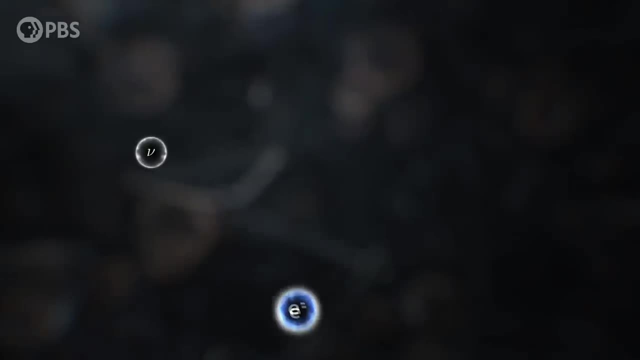 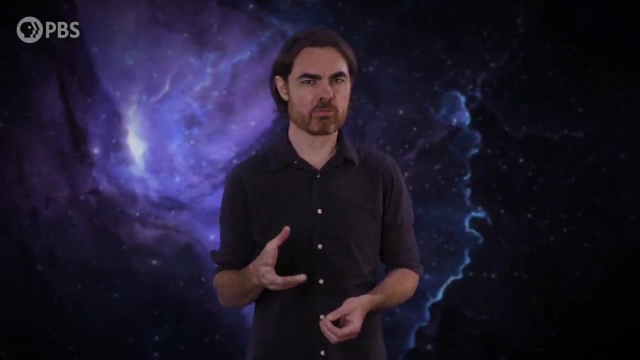 can speak the language of that force. The force of gravity is a sort of lingua franca, a common language that every particle with mass can speak. But gravity is a little different to the other forces. it's not part of the standard model and we just don't know what it is. So we're going to talk about gravity. 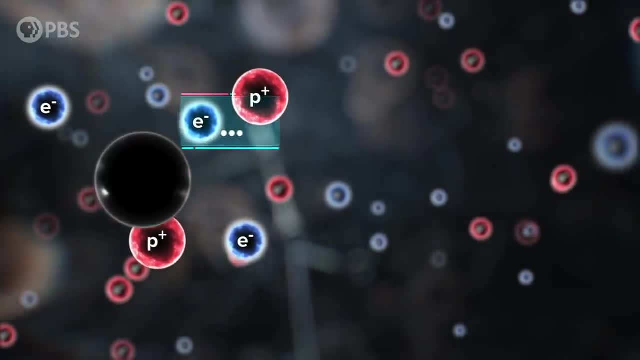 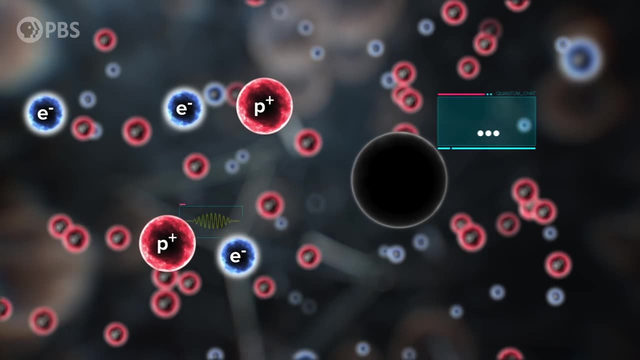 in a bit. But we don't even know if it has a quantum field. The main requirement for a dark matter particle is that it doesn't speak electromagnetism. It doesn't produce light, hence the dark part, But it also doesn't absorb light otherwise. 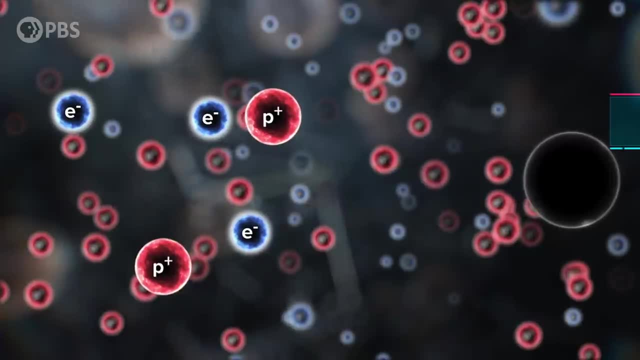 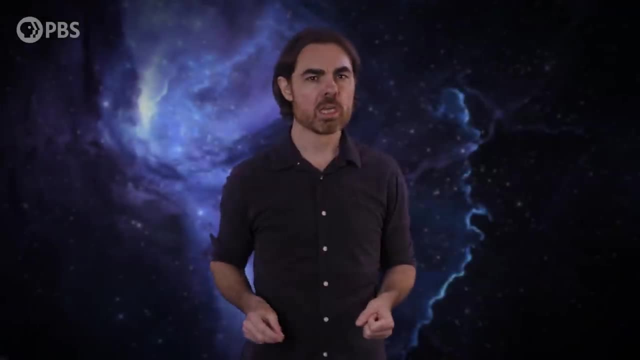 we'd be able to detect it when it blocked light from the more distant universe, in the same way that we see the black lanes of dust that block light from the center of our galaxy. No dark matter is both perfectly dark and perfectly transparent. Good, so it must be. 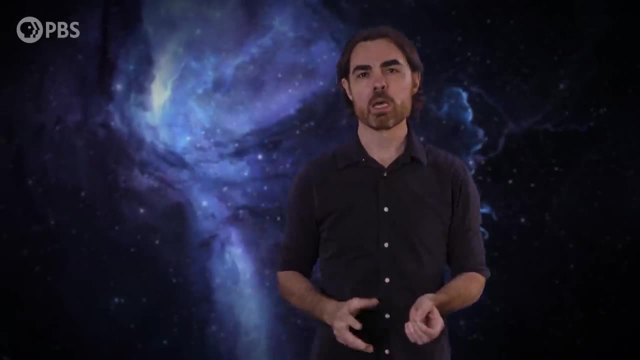 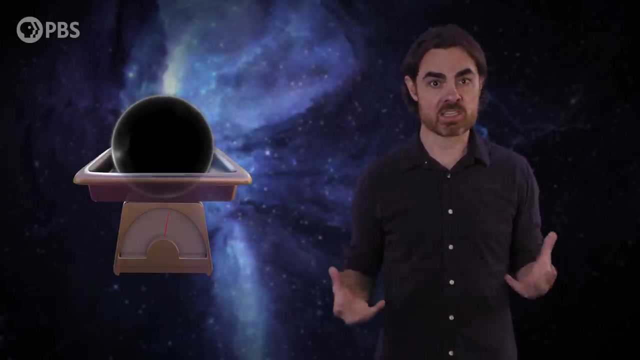 electrically neutral. Like it can't be completely transparent, it can't be perfectly neutral. Dark matter can't have charge, but it also must have mass, because the only thing we've ever actually seen dark matter do is to exert its gravitational influence. Dark matter speaks. 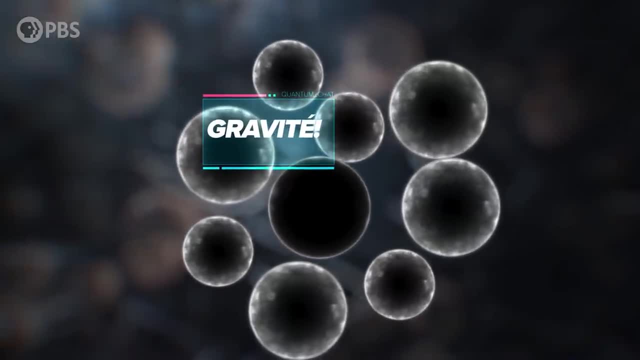 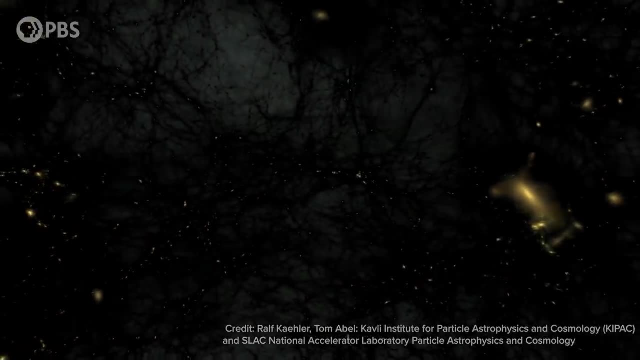 gravity, And we can learn an awful lot from how it exerts its gravity. We can map where dark matter is found by how it affects the rotation of galaxies and how it drives the orbits of galaxies inside galaxy clusters, and by the way it bends light around. 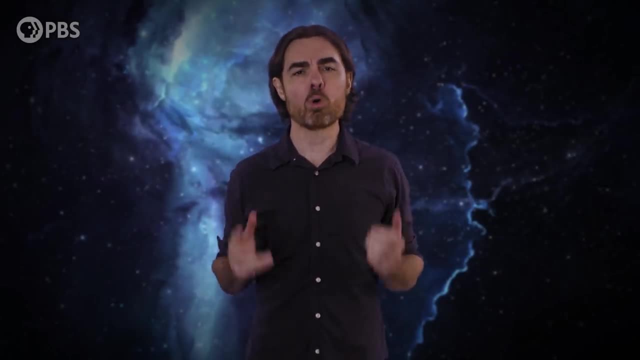 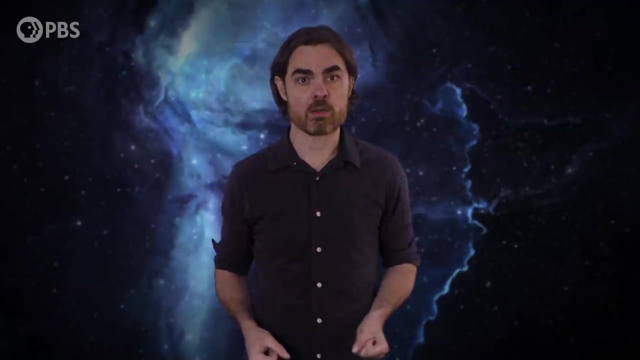 galaxies and clusters. These tell us something really important: Dark matter is far more spread out, more diffuse than almost all of the visible matter, And that tells us a lot about any prospective dark matter particle. For one thing, dark matter doesn't tend to interact with itself. 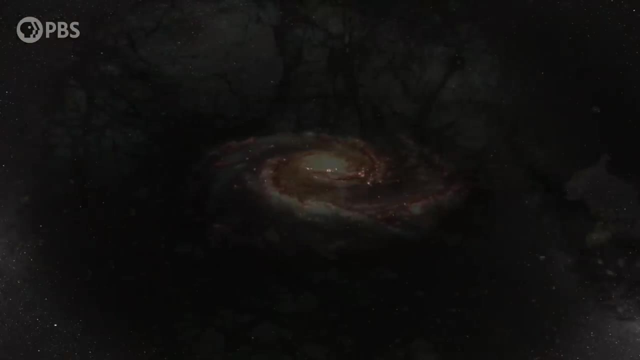 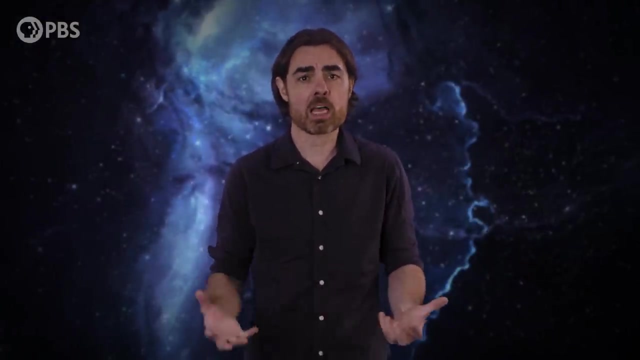 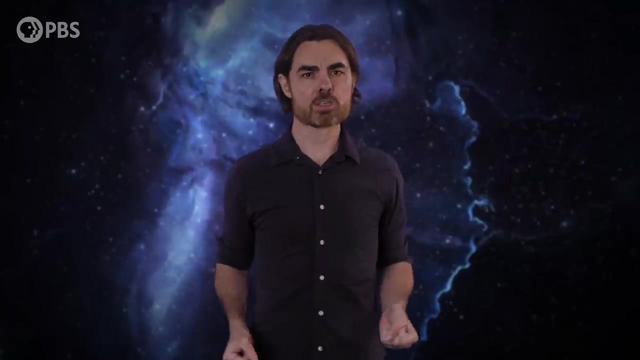 – at least not very much. If it did, then giant regions of dark matter would lose energy in those collisions and contract. They might collapse into dark matter galaxies or dark matter stars or dark matter people, But no. Dark matter seems to stay puffed up in gigantic halos surrounding the much more 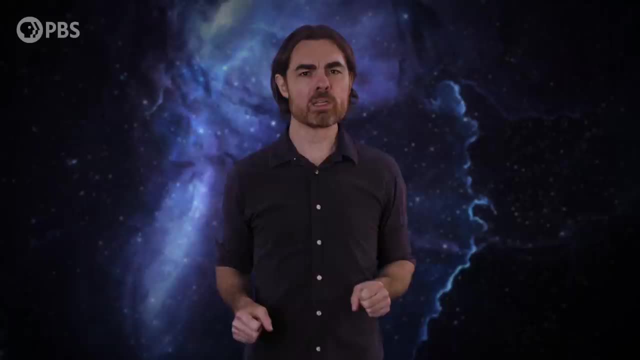 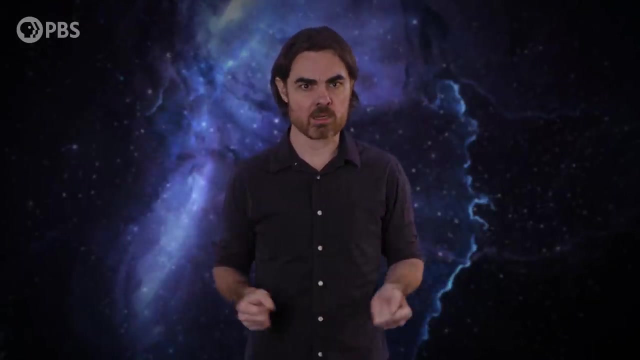 concentrated clumps of visible matter. In fact, galaxies are really just shiny dustings of stars sprinkled deep in the gravitational wells of massive reservoirs of dark matter. But the fact that dark matter forms those giant halos at all tells us something very 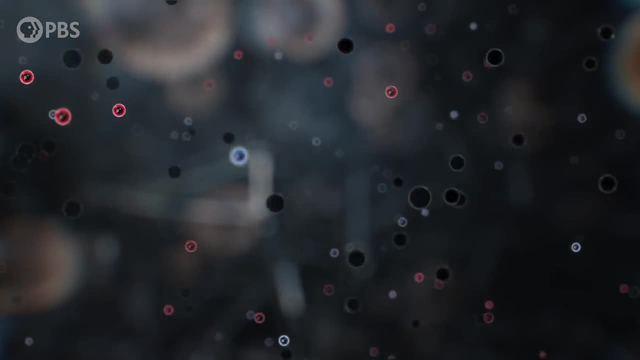 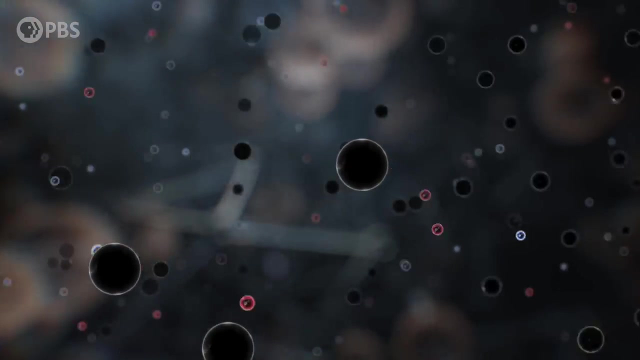 important. It gives dark matter a temperature. Well more accurately, it tells us how far dark matter particles would go. We're able to travel in the early universe. This free-streaming length of dark matter is how far a dark matter particle could travel before interacting with something – typically. 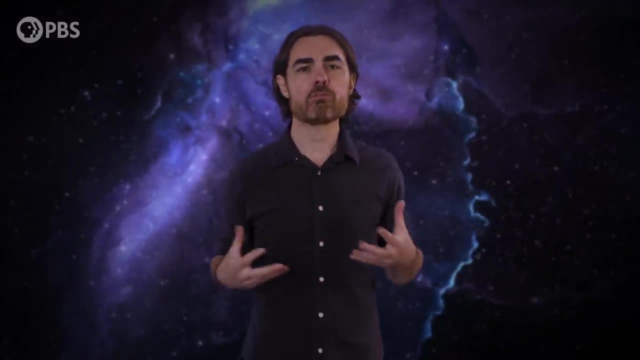 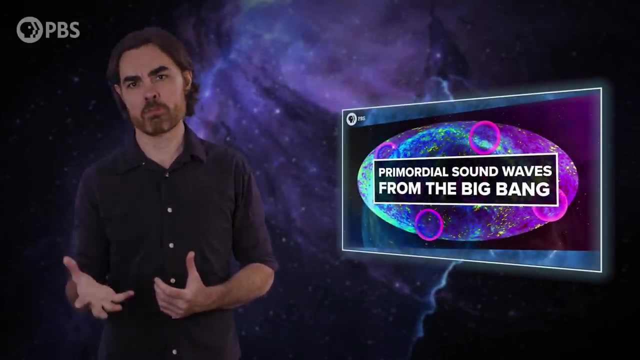 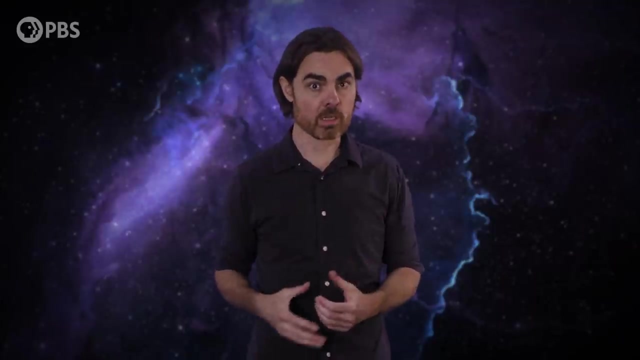 another such particle In the early universe. that distance influenced the size of the seed structures which galaxies would later form from. We've talked about that structure formation before Now. based on how that structure did end up forming, it seems likely that dark matter was moving pretty slowly. We refer to such 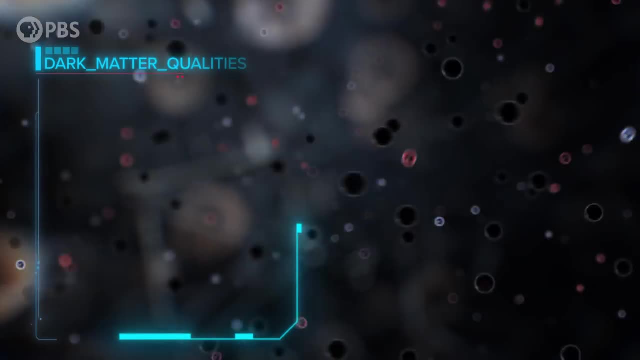 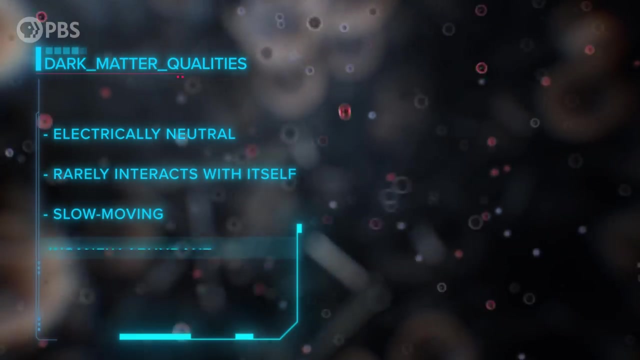 dark matter as coli. So let's review. If dark matter is a particle, it's electrically neutral and doesn't interact much with itself, and it's relatively slow moving and also insanely abundant. For a long time, people thought the neutrino might be dark matter, being neutral and the most abundant known. 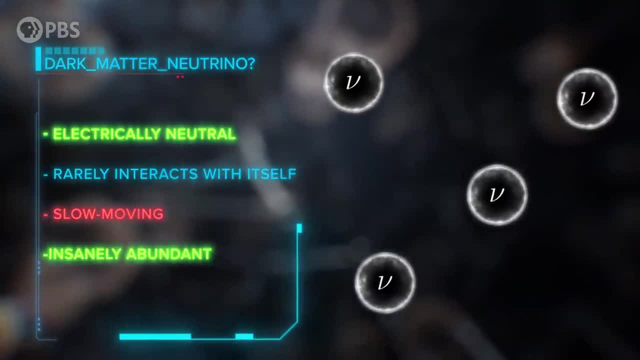 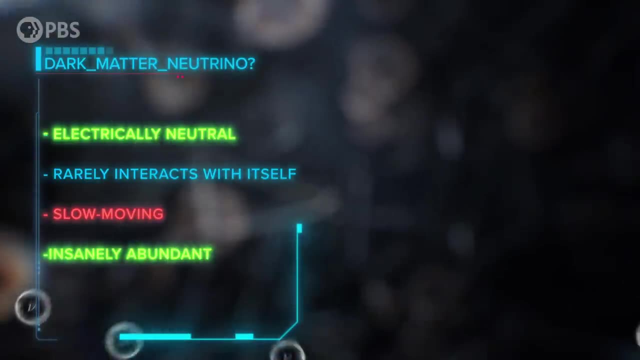 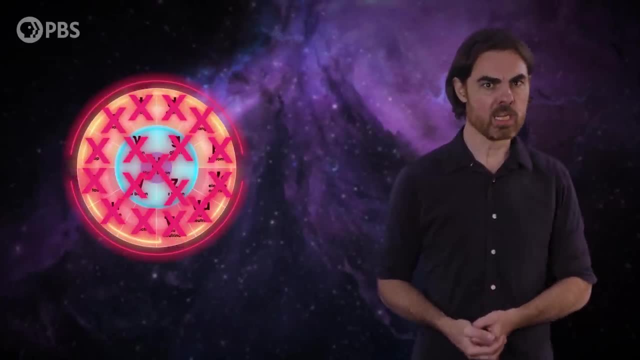 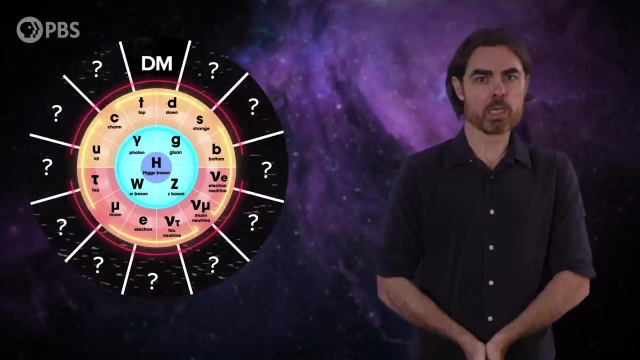 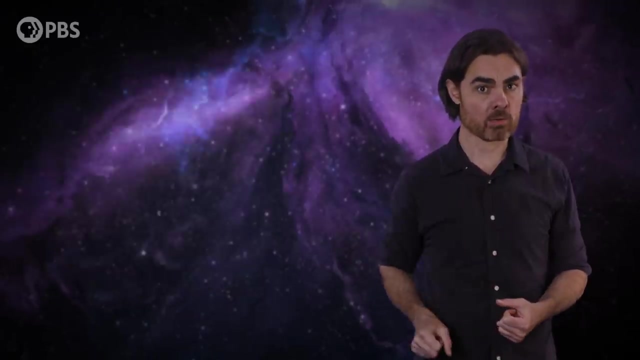 So it seems like dark matter just works, which sounds annoying but actually gets physicists rather excited, Because discovering a dark matter particle maybe our best bet for finding a bigger, deeper theory beyond the standard model. It would also be a No-brainer Nobel prize, and many researchers have devoted their lives to hunting down this particle. 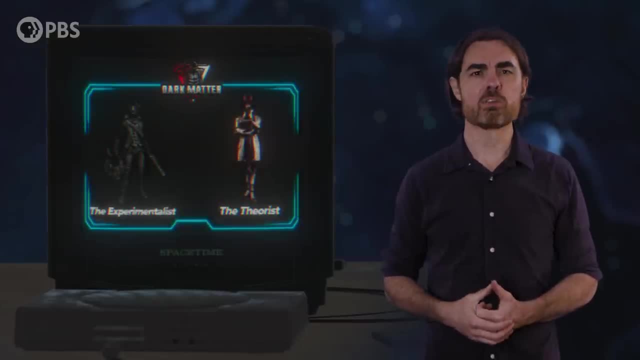 Dark matter hunters come in two breeds. One type searches for new evidence out there in the universe or in our particle experiments here on earth for evidence of particles that don't fit the standard model. The other type delves deep into theory, in the speculative mathematics beyond the standard. 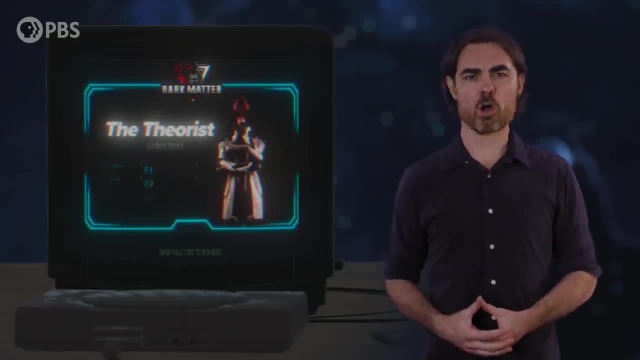 model for signs of new particles. Today we're going to focus on the theoretical prospects, because we might as well have some fun before those pesky observations ruin everything with their facts. Actually, we don't have to go too far beyond the standard model to find our first dark. 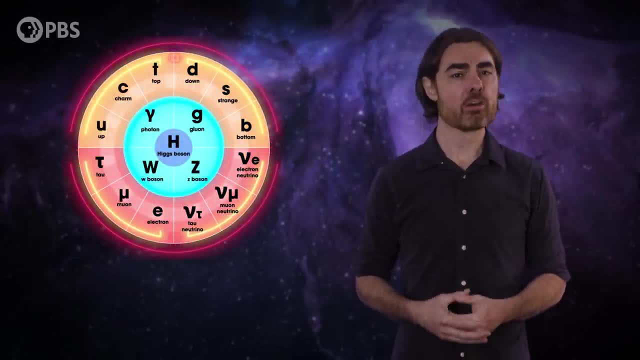 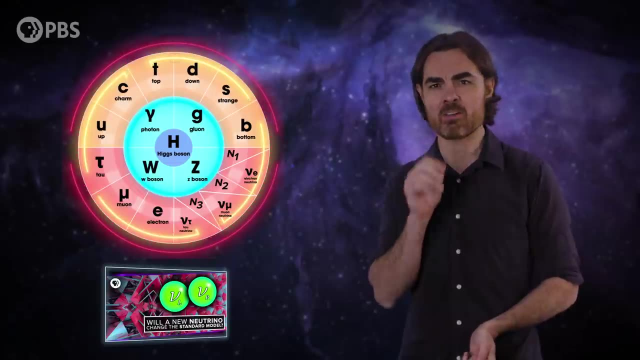 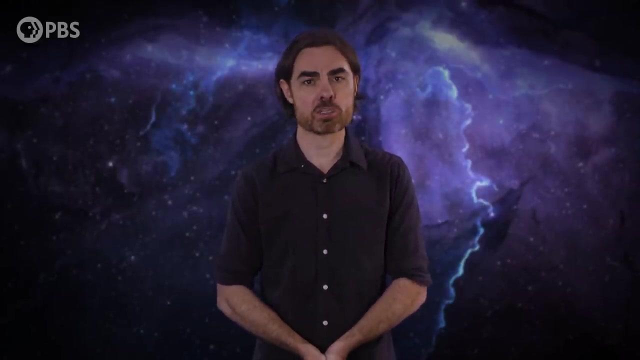 matter candidate. Completely independently of our quest for dark matter, physicists have hypothesized a new type of neutrino, the so-called sterile neutrino. I won't describe these in detail now because we've been over them before, but, in short, as ghostly as neutrinos are sterile, neutrinos are far ghostlier. They don't even interact by the weak force, which means they're almost impossible to detect. There are some exceedingly clever experiments to do so, like we saw that time we visited Fermilab. If sterile neutrinos exist and are massive and slow-moving enough, they are a great dark. 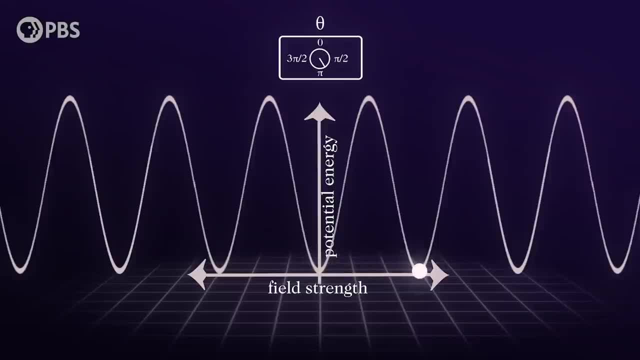 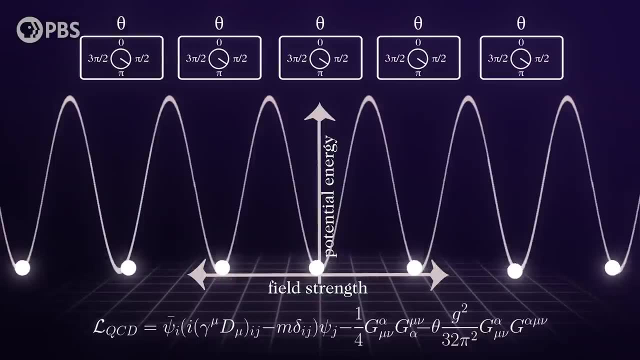 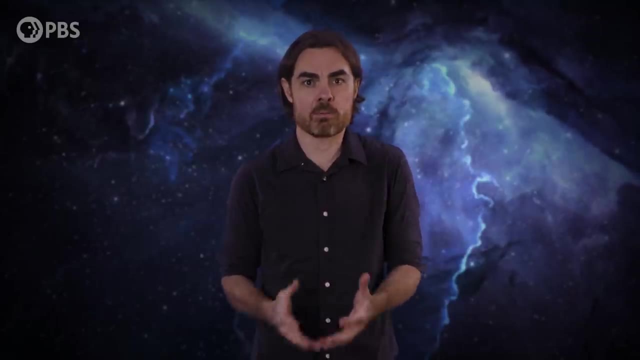 matter candidate. Another candidate that we've discussed before is the axion. This is a weird little particle that popped up in the math when physicists were trying to solve another mystery of physics, the so-called CP problem. Axions, if they exist, would be incredibly light, maybe 1% or less the mass of the already puny. 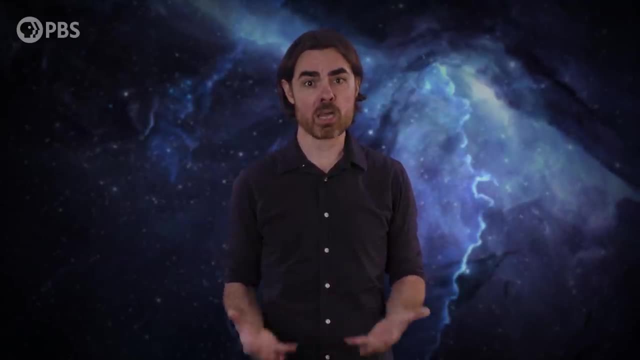 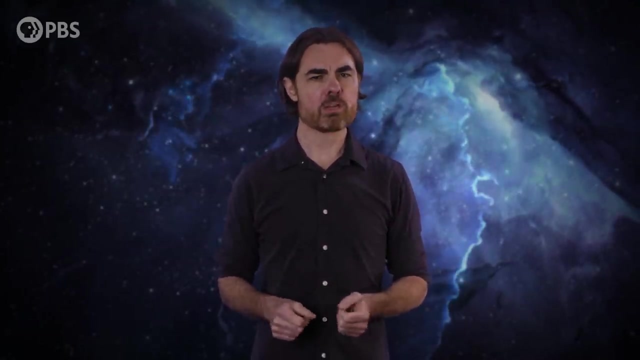 neutrino. So to account for dark matter, they'd need to exist in prodigious numbers, But according to pro-axion physicists, that may well be the case. OK, So the things we've already talked about- Explorations of the theoretical landscape- have led physicists to multiple possibilities. 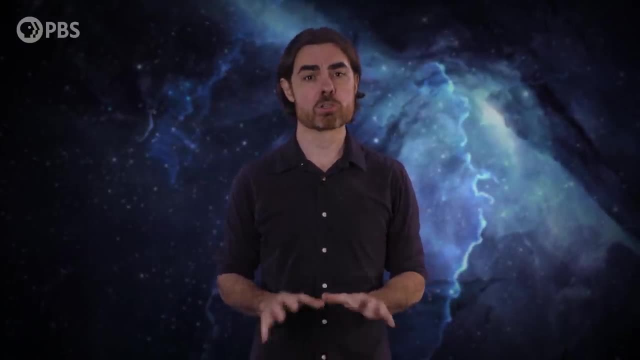 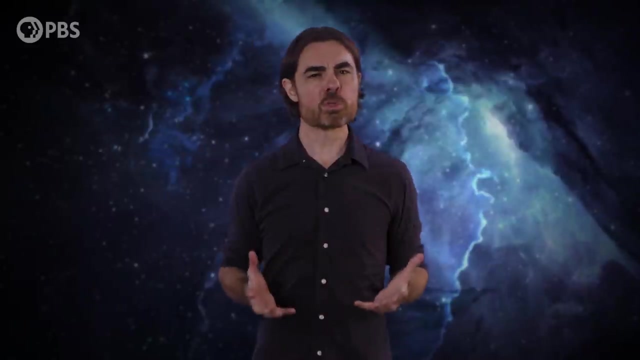 for dark matter particles. One of the most promising ideas comes from supersymmetry. We have already talked about supersymmetry, but not about how it could give us dark matter. Supersymmetry is an extension of the standard model and it proposes that all the regular 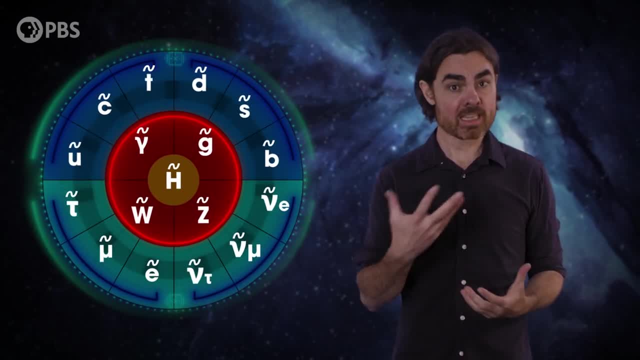 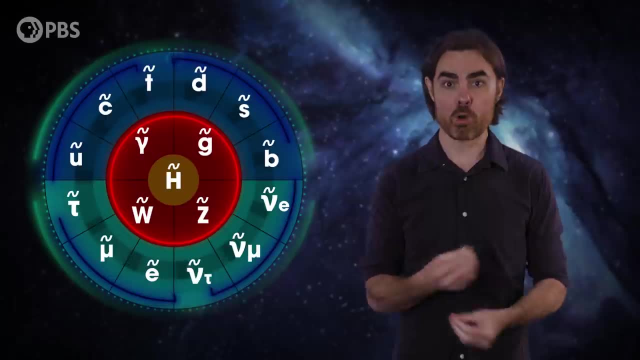 particles, both matter and force carrying, have twins counterparts on the opposite side of the table. Every matter, particle or fermion has a supermassive mass. That's what we're talking about. Every particle has a supersymmetric force carrier or boson, and every boson has its 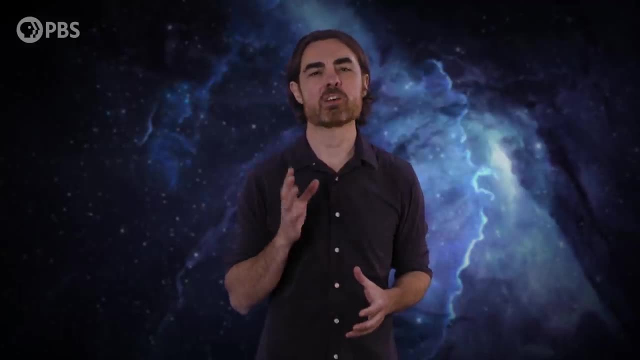 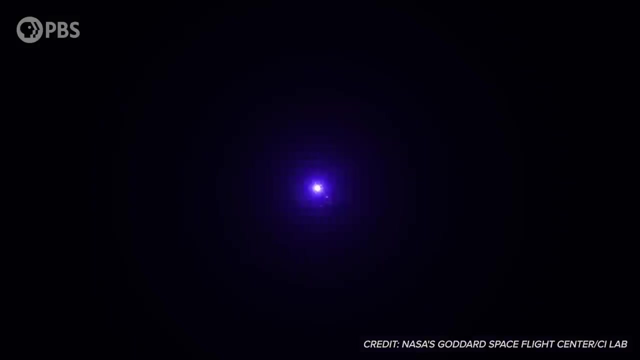 fermion twin. It's expected that these supersymmetric particles are much heavier than their standard model counterparts, And that may explain why we haven't seen them in our particle accelerators. perhaps we just haven't produced enough energy to make one yet, But they may have been produced in the insanely energetic early universe and the leftovers. 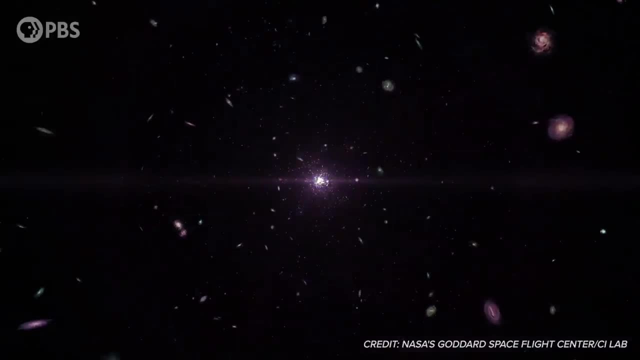 from that time could still be throwing their weight around, so to speak. The simplest kind of dark matter that we get from supersymmetry is called a neutralino. It's a sort of three-in-one particle where the electrically neutralized energy is the 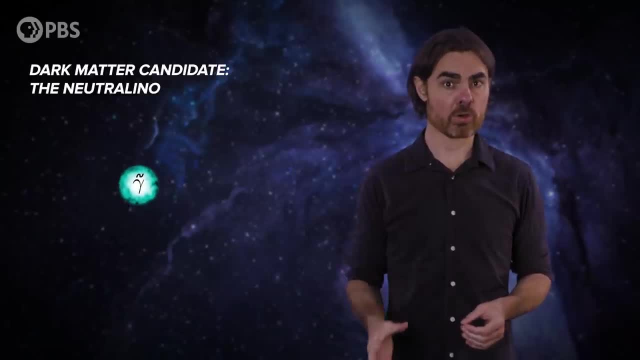 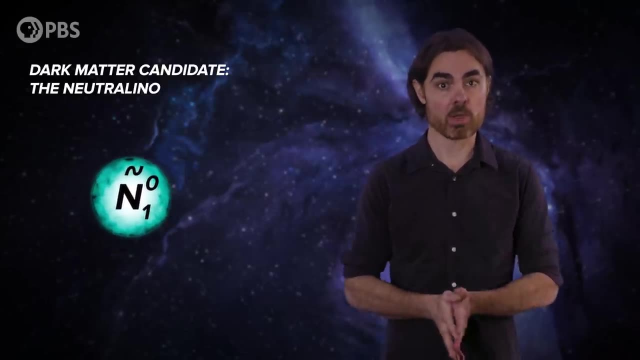 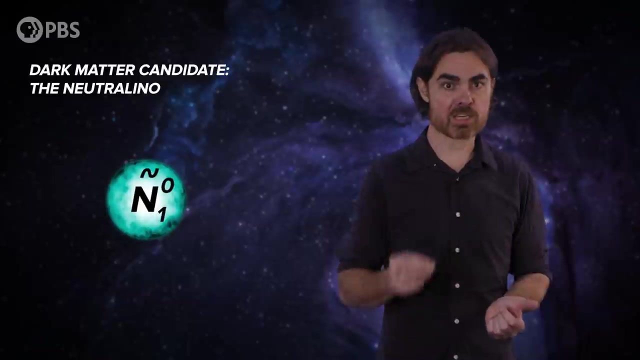 superpartners of the z-boson, the photon and the Higgs particle all mixed together. In some models these are the lightest supersymmetric particles possible- LSPs- but they're still incredibly heavy And while normally heavy things do tend to decay into lighter things, if these can't, 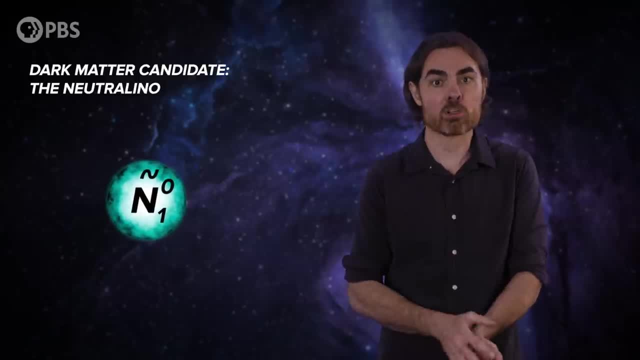 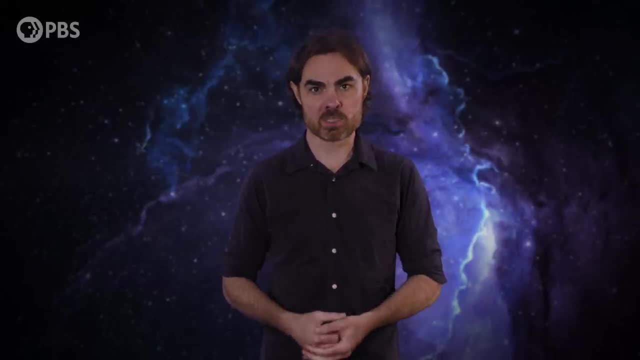 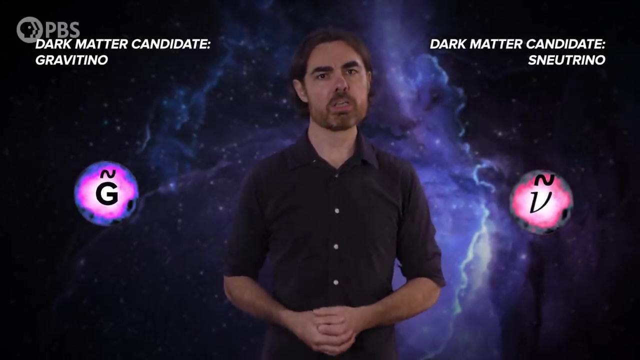 decay into stanton-bottled particles, then they'd be stable and long-lived, an almost perfect dark matter candidate. There are other dark matter candidates in different flavors of supermassive energy, for example the counterparts of the neutrino or the graviton. 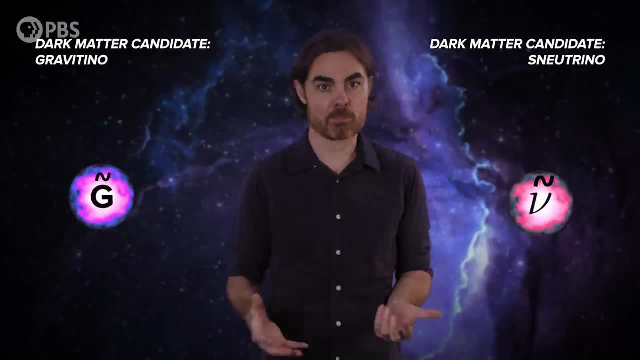 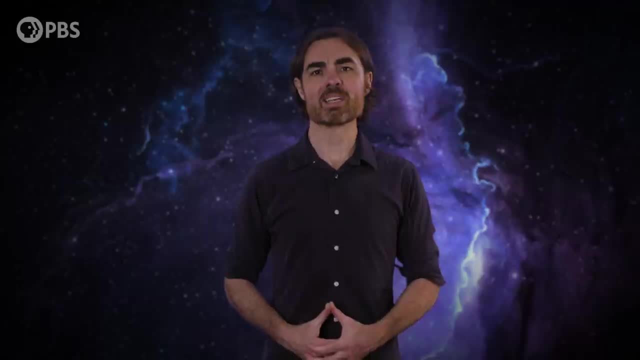 The expected mass of these particles is eerily close to the mass expected for a certain type of dark matter, which some would say is a point in favor of supersymmetry. This seeming coincidence is sometimes called the WIMP miracle, but for that to make sense, 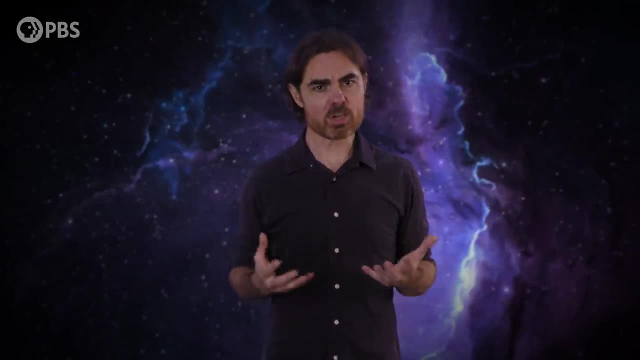 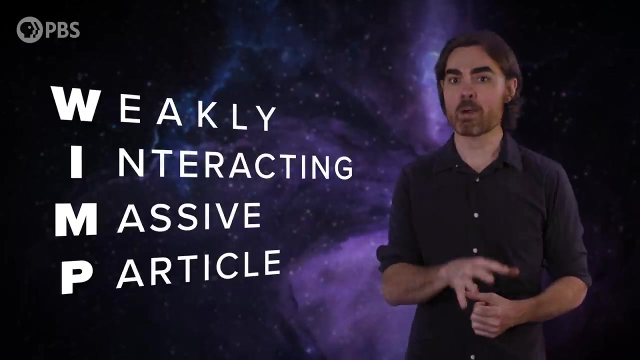 I guess I should explain what a WIMP is. Supersymmetric dark matter particles like the neutralino are examples of a general dark matter particle type called the WIMP or weakly interacting massive particle. The idea of the WIMP was proposed independently of any actual WIMP candidates. 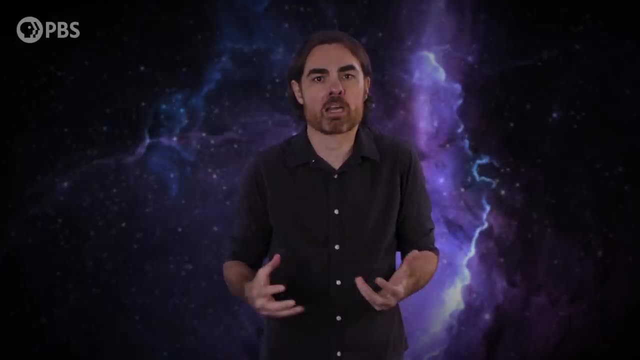 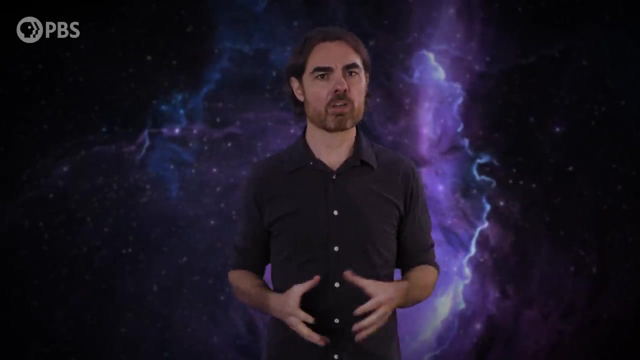 It's a description of what some physicists thought dark matter particles had to be like, which is to say weakly interacting and massive. The massive part is obvious enough. It helps if you want to make up 80% of the mass in the universe and it also slows the 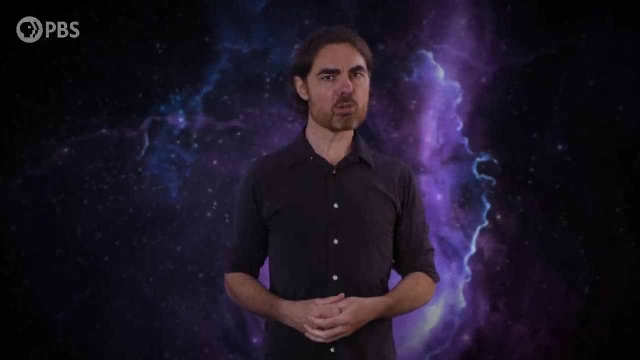 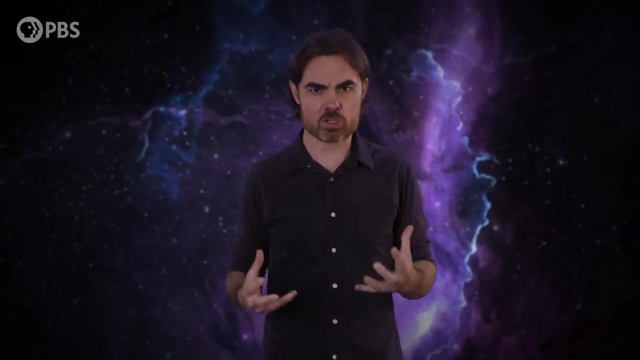 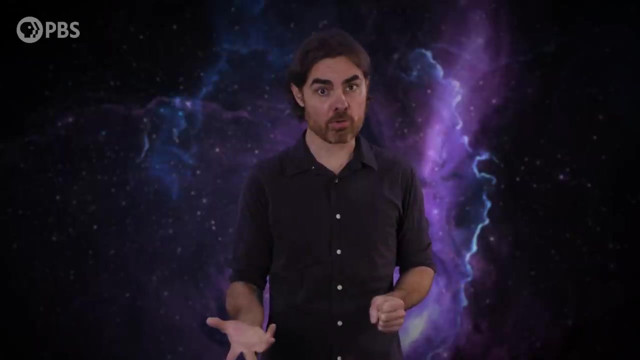 particle down. It helps make it cold. We also covered weakly interacting. It helps dark matter halos stay puffed up. But it also turns out that interaction strength of dark matter is incredibly important. It may have governed how every interesting thing in our universe first formed. 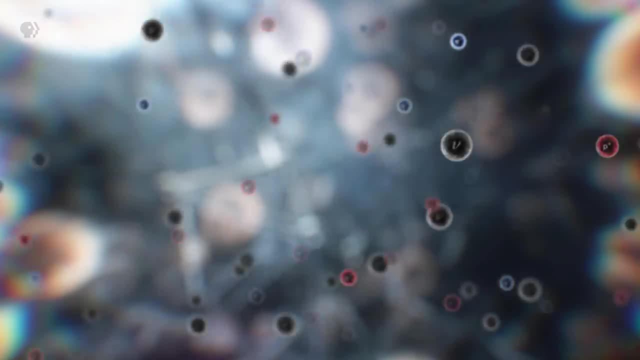 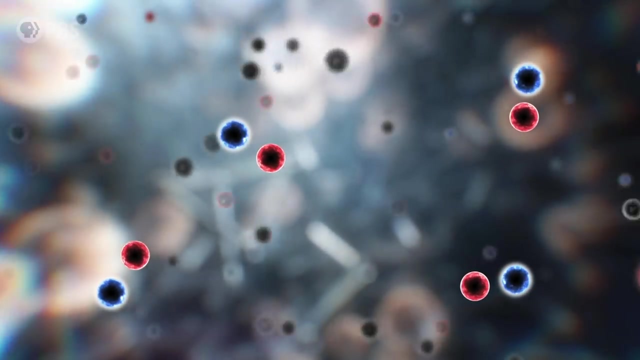 The idea is this: In the first fractions of a second after the big bang, particles and their antimatter counterparts would have been popping into existence, constantly borrowing energy from the crazy radiation of that time, And then, when the particle bumps into existence, it's gone. 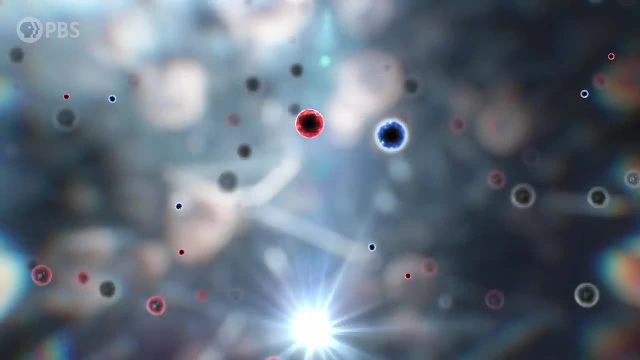 And then when the particle bumps into existence, it's gone. When the particle loops the natuur, they release active energy, Unable to react the antiparticle cool effect it yüked as it may have been approaching its solution. And when that target pops into its antiparticle, they both annihilate, releasing that energy. again. As the universe cooled and energy dropped, that process ceased. We were left a universe full of particle-antiparticle pairs that would just have been annihilated over time. But it's possible. particles may not have been able to find an antiparticle counterpart. 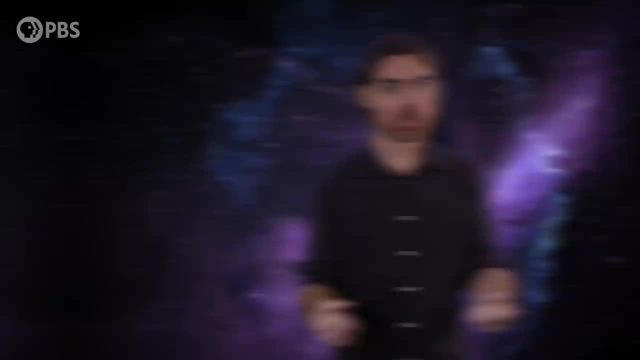 before the expanding universe pulled them too far apart. Now, things like electrons and anti-electrons – or positrons – interact very strongly via the electromagnetic force. we've seen a possibility for when our weak absorbance ofерх forming horas foreفسbresumbah. 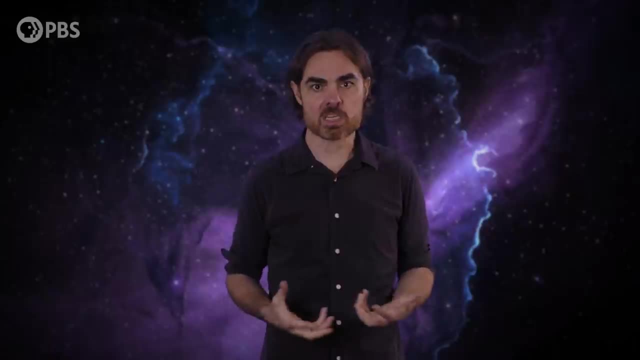 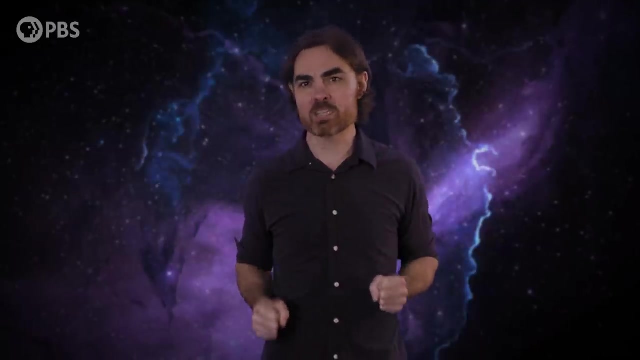 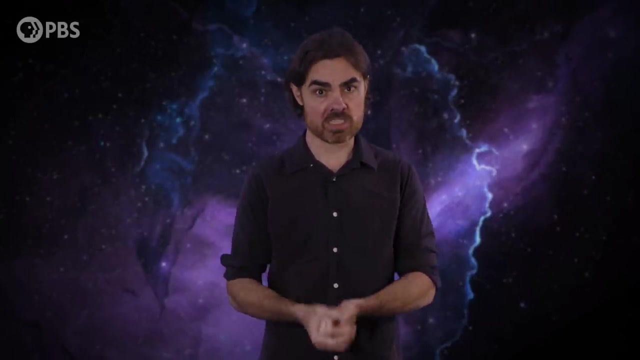 Which means they find each other too easily. The universe didn't expand fast enough to throw these particles apart, and so almost all annihilated. But a WIMP, with its extremely weak interaction, would more easily dodge its antimatter buddy, and so countless may have survived to this day. 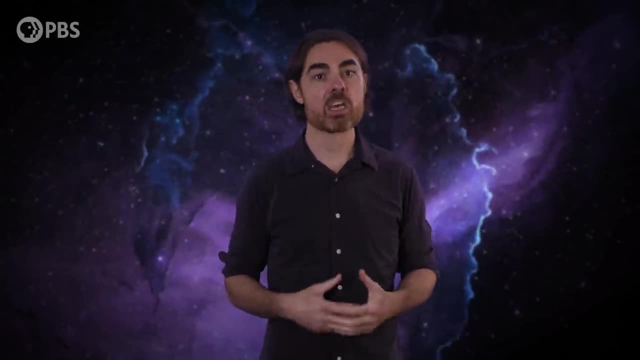 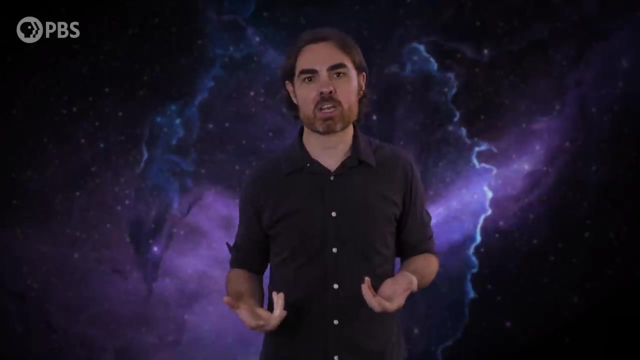 So it turns out, you can do a calculation of what interaction strength such a relic particle would need to have in order to survive in sufficient numbers to give us dark matter, And that interaction strength is about the same as the weak interaction. ergo, WIMPs interact. 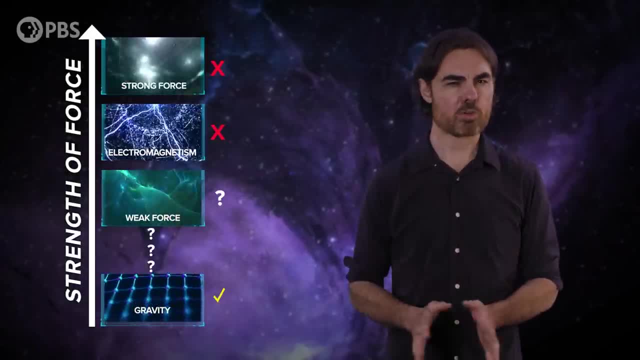 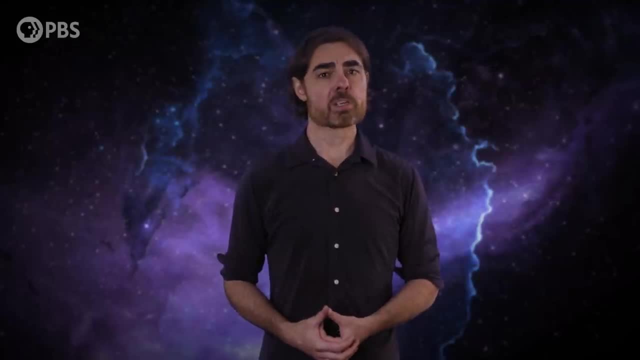 by the weak force only or by something weaker? OK, so we have multiple possible members of the dark sector, and we didn't even cover all of them. Perhaps none exist, but perhaps several do. It's possible that an entire ecosystem of particles are going about their dark business. 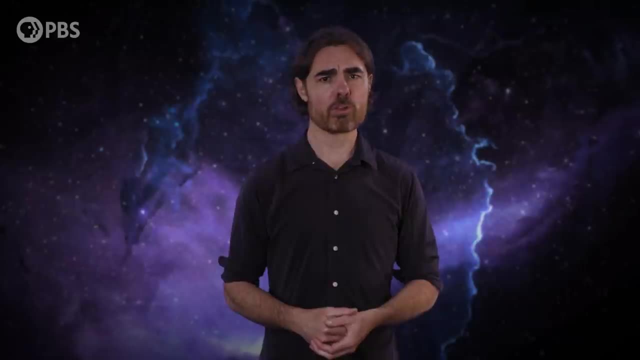 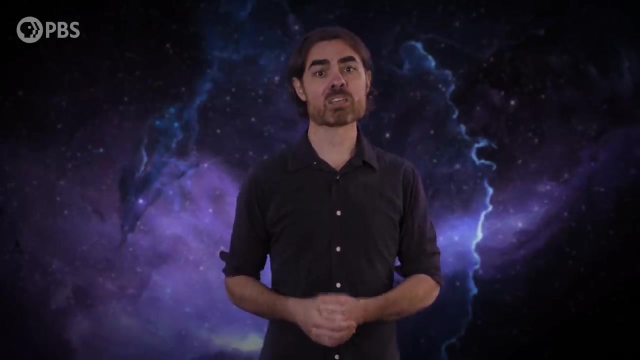 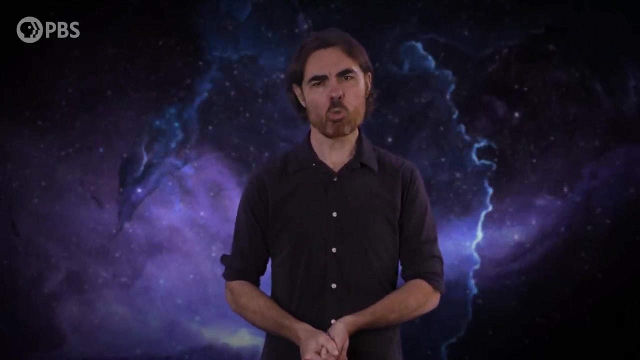 across the universe, interacting by dark forces, all of them oscillations in their own dark quantum fields, Perhaps with their own complexity and diversity, Because dark matter is weakly interacting. our light sector is probably more complex, Probably, But to know one way or another, one of the many brilliant experiments currently in progress. 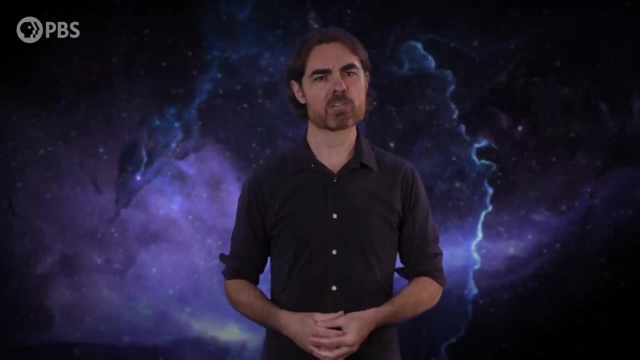 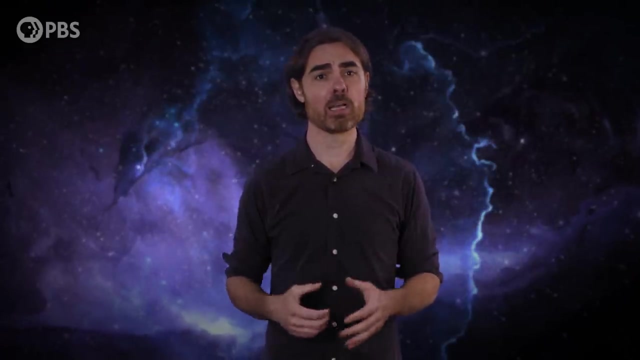 or planned, will need to bear fruit. We'll talk more about those experiments another time. For now, we'll just have to enjoy knowing that our lightweight light sector exists in parallel to this completely invisible and vastly more massive sector. But that's not all. 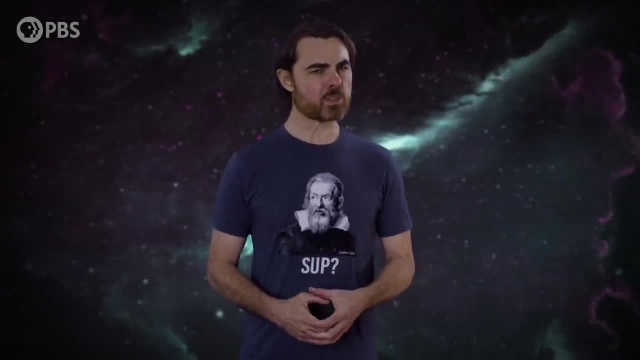 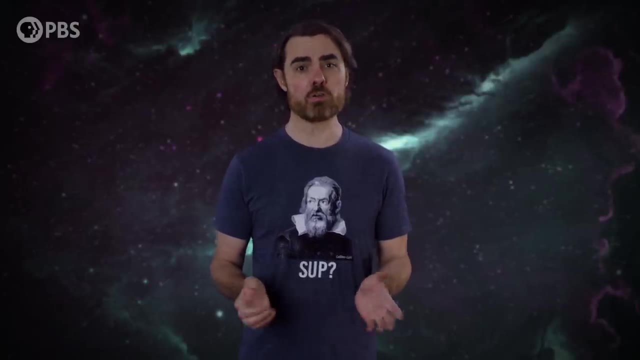 We'll talk more about dark space time Before we get to comments. we just wanted to let you know that, while we love talking about space, if you have more earthly concerns, you should check out PBS Terra on YouTube and their show Weathered. 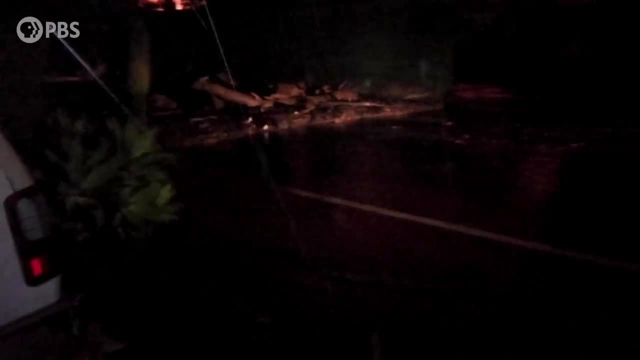 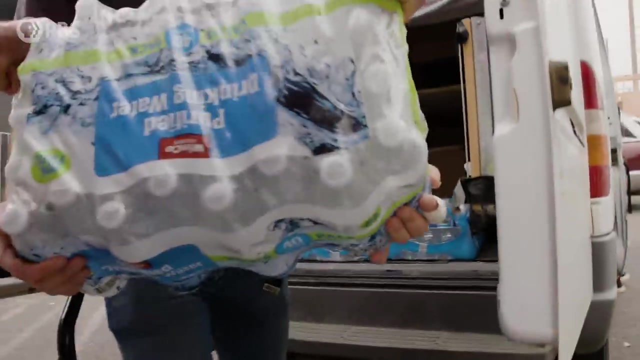 Here is a quick trailer. Are you prepared for the next disaster? The flash flood's right there. Keep going, keep going, baby, keep going. Are you ready to help your family and neighbors? Welcome to Weathered. In this show, we'll explore the most pressing natural disasters in the US and around the 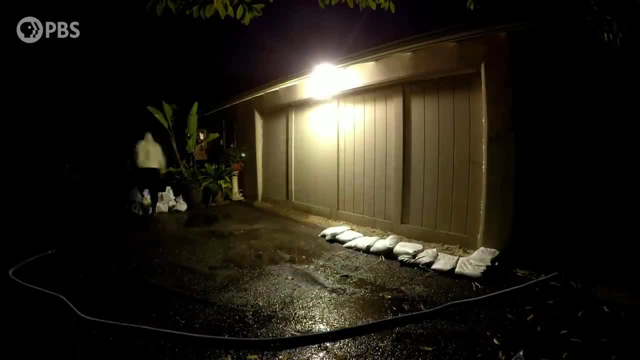 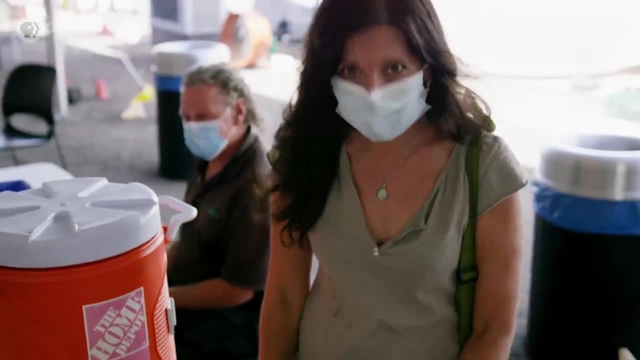 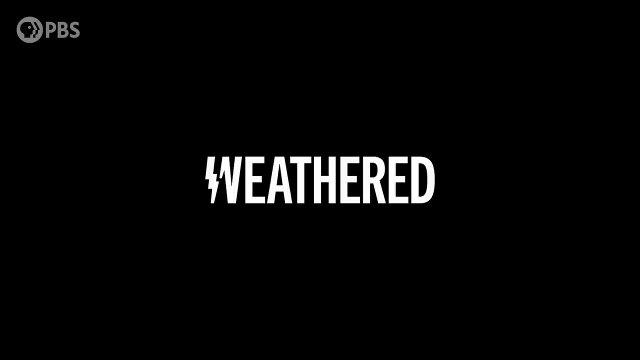 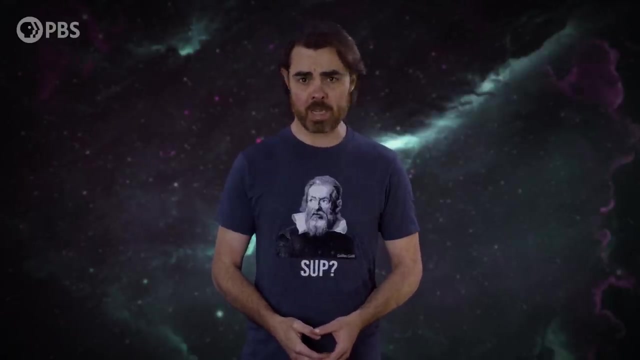 world, How they're changing and how you can prepare. This is literally a lifesaver Like this saves people's lives. In the last episode, we asked the question that I know all of you have had on your minds: Would a spaceship traveling near the speed of light cause a closed universe to contract? 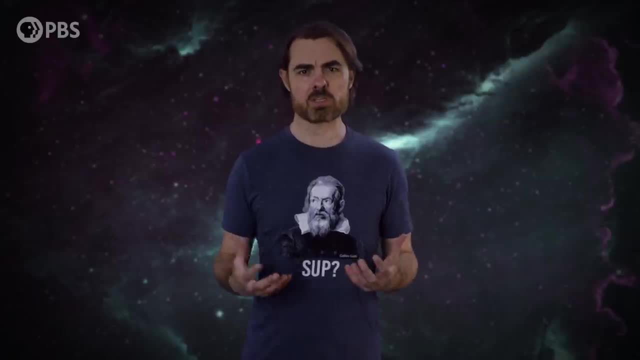 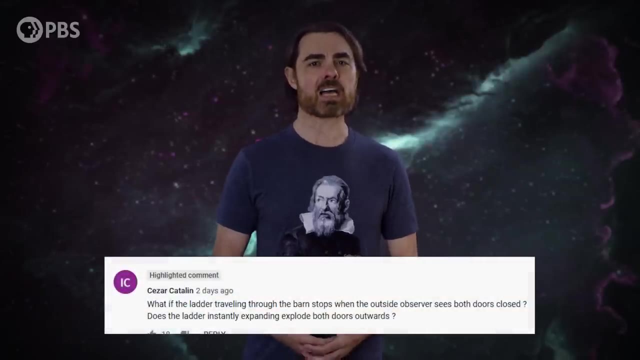 so much that it would smash into its own ass. Let's find out In the process of answering that. we explored the Ladder Paradox and the Twin Paradox, And that's what our questions are about today. Cesar Catalan asks: what if the ladder traveling through the barn stops when the outside observer? 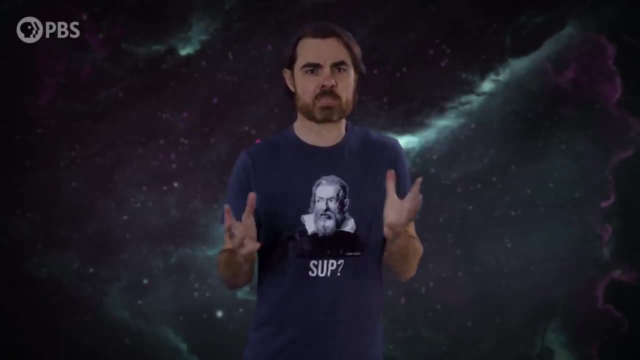 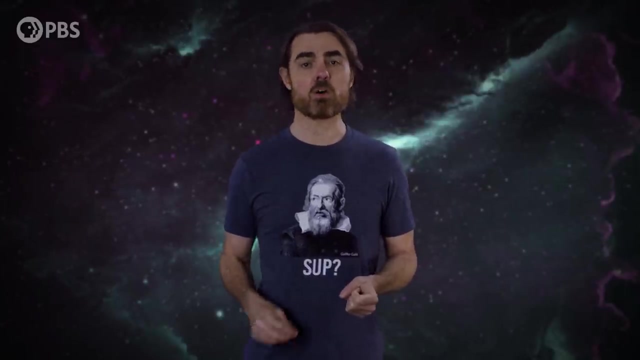 sees both doors closed, Does the ladder instantly expand, exploding both doors outwards? That's an awesome question. The answer looks different depending on your reference frame. From the frame of the barn, the ladder is fully inside And the exit door remains closed. 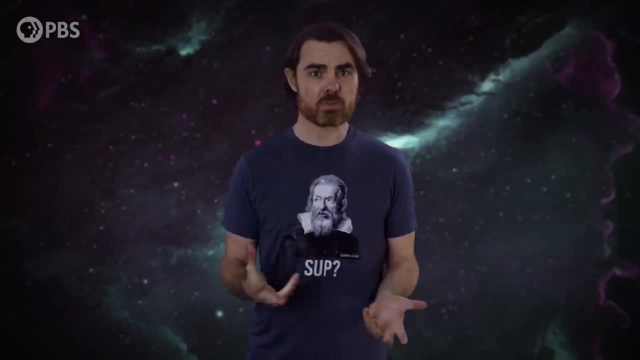 Let's say it's an adamantium barn door. The ladder collides with the door at a high fraction of the speed of light and a shockwave blasts down the length of the ladder, totally destroying it and embedding the walls of the barn with splinters. 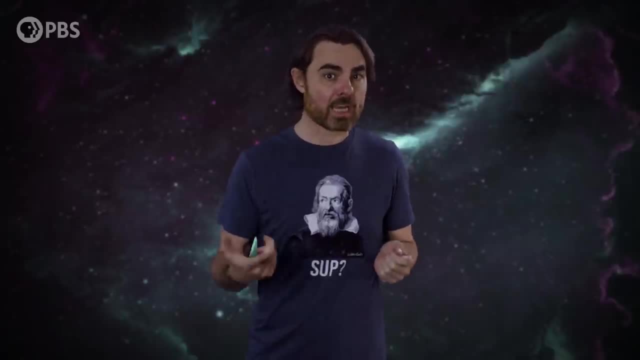 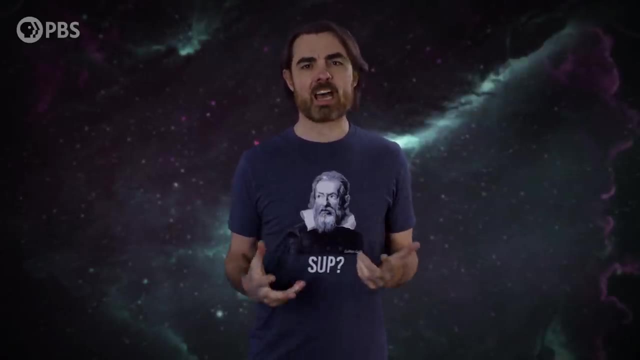 And all those splinters have to be inside the barn. From the ladder's perspective, its butt is still outside the barn when its front end hits the door. There's an absolute limit to how fast that impact could communicate itself down the ladder. The shockwave can go no faster. 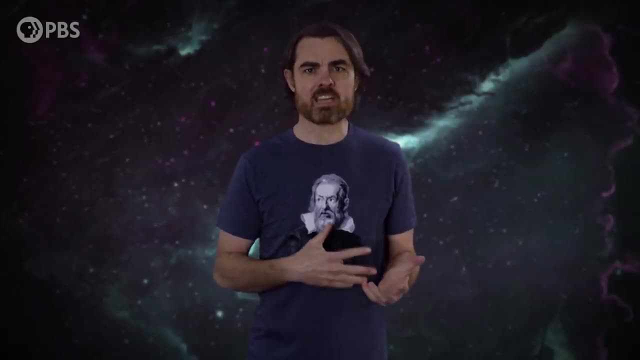 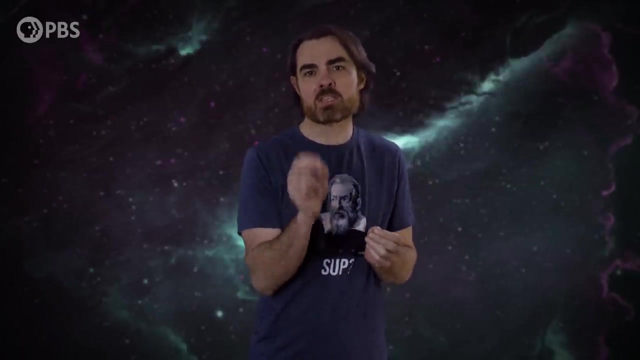 So by the time the base of the ladder even knows that anything at all has happened to the front of the ladder, it's already inside the barn. The shockwave hits the base of the ladder at the same position in the barn, from either the ladder or the barn's point of view. 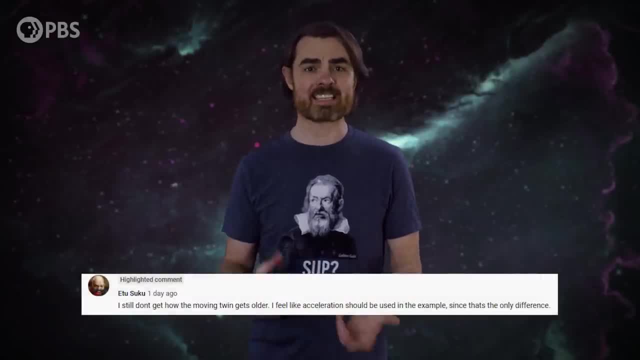 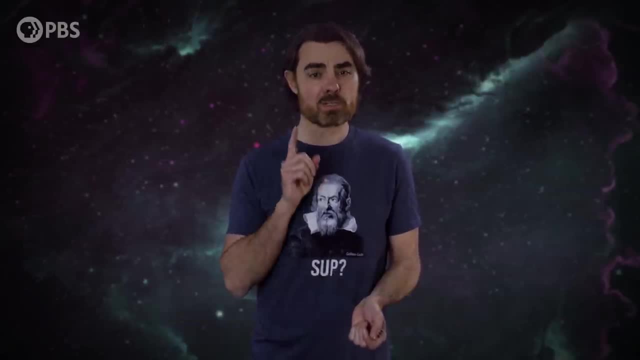 Etusuku points out that the difference between the traveling and stay-at-home twin is actually acceleration. so shouldn't acceleration be used to account for the time difference? Well, I'm actually glad you mentioned that. Yes, The ladder needs to decelerate and then accelerate again to turn around. And according to Einstein's equivalence principle, acceleration is fundamentally the same as gravitation as far as the laws of physics are concerned. So can we apply gravitational time dilation to the traveling twin as though they were standing on the surface of a planet with the same gravitational acceleration? Yes, we can, And we'd get exactly the same answer as if we just have the traveling twin instantly flip its velocity around with no slowing down or speeding up. It turns out that there's no distinction between all the types of time dilation. as far as the universe is concerned. 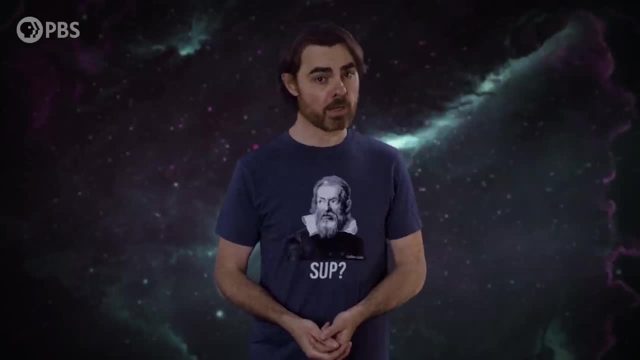 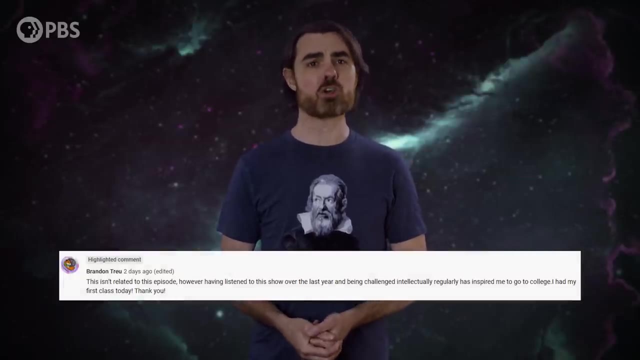 And that's something we really do need to explore more carefully. in an episode coming very, very soon, Brandon Treyu says This isn't related to the episode. however, having listened to this show over the last year and being challenged intellectually regularly has inspired me to go to college. 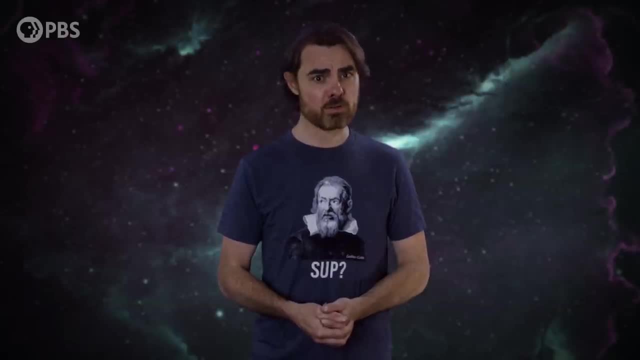 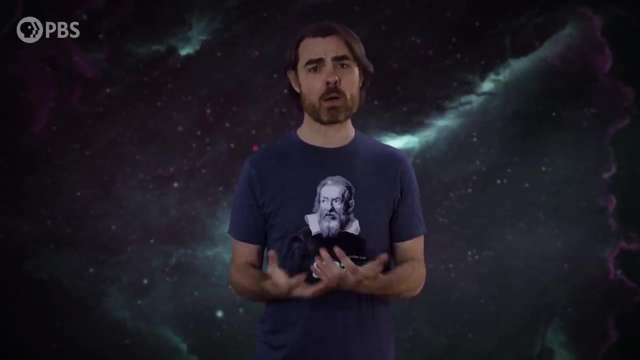 I had my first class today. Well, Brandon, thank you for sharing this. This is exactly the kind of feedback that keeps us doing this show. If we played a small part to inspire you to embark on this new adventure, then it's all been worth it.